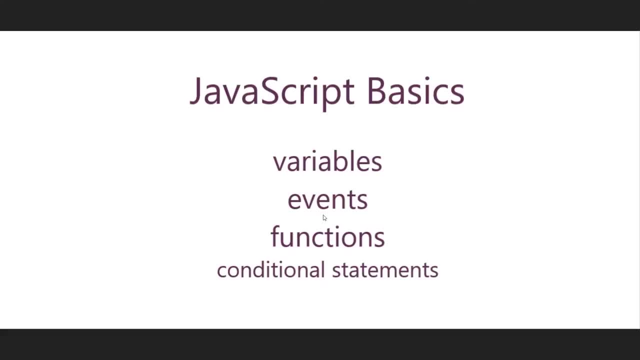 page that JavaScript can then react to, or you can attach some functionality to different events, And then functions are a way to put a bunch of code into this function which you name, and then you can refer to it in your code a bunch of times or here and there. 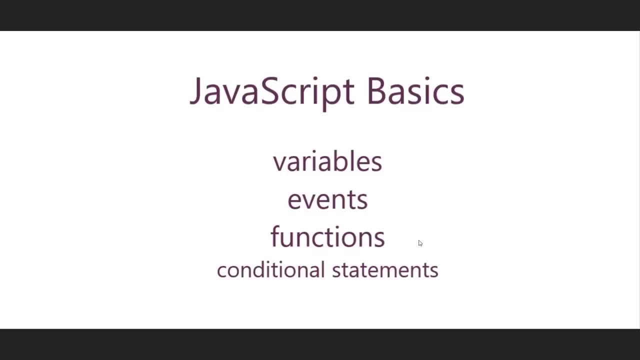 or attach it to events. And again, it's another way to prevent repeating code and refer to a functionality with just usually a semantic name that makes it clear what is going to be doing. And I'm going to touch on conditional statements, which are usually part of functions, So conditional. 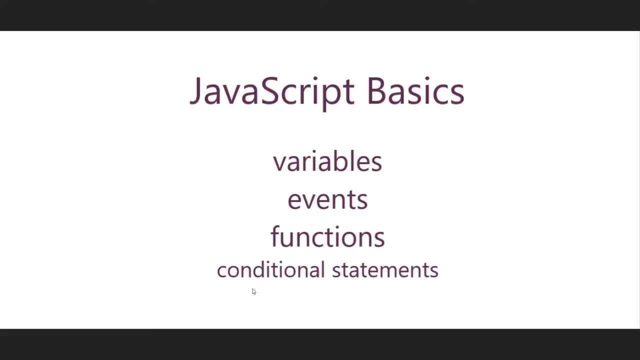 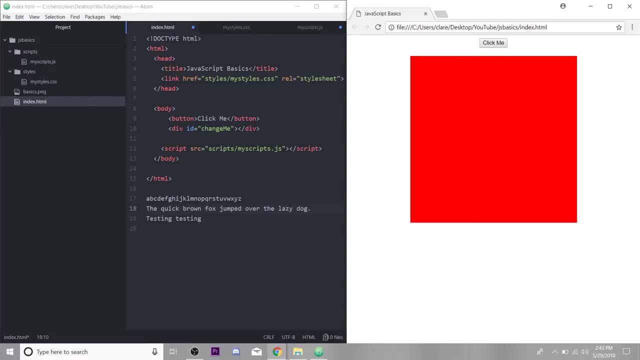 is just if else. So we're going to test a condition. So if something is a certain way, do this else, do something else, And this will again make sense as we get going. Okay, Okay, Okay, Um, so this is just a little page I put together. You can see in the markup: here we have a 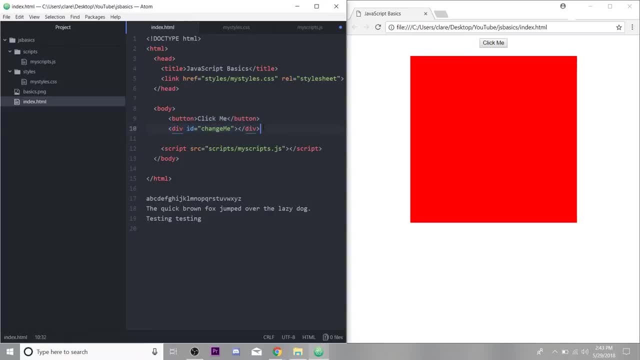 button and we have a div with the ID of change me and then over here: Okay, And then you see, we link to this style sheet which is just targeting this change me div, making it a square, giving it a little bit of a margin, um, centering it and giving it a background. 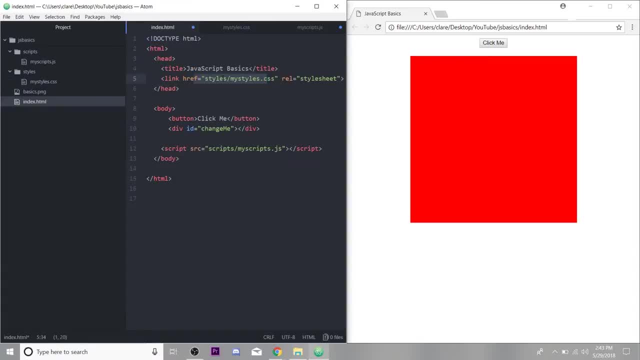 color And I just um centered everything on the page And then down here at the bottom. this is something new. this is a script tag where we are linking to an external myscriptsjs file, javascript file- which over here, is empty, and you load a script at the bottom of your body tag, as opposed to in the 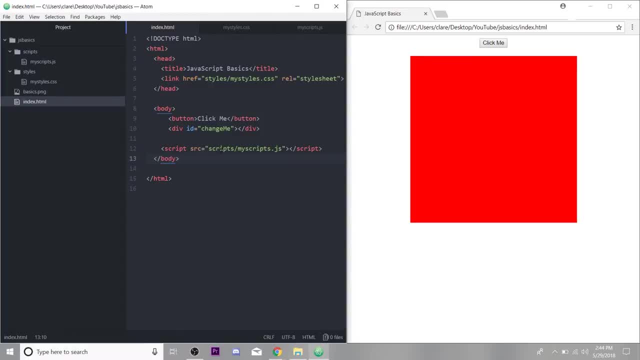 head tag because typically you're going to be referring to your html down here and some javascript will load with the page and you want it to be after things that it's referring to. so just a standard practice to load your script in the bottom and it uses a source attribute as: 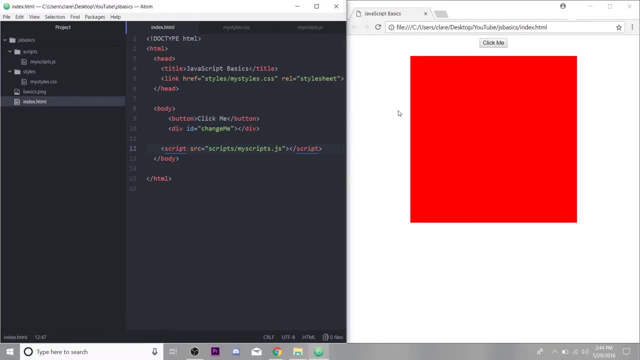 opposed to href. but here's our page. it's just a non-functional button with a box. so, to get started, we're going to assign some variables in our javascript file and the way you declare a variable is just var and then the name of the variable. so let's do a variable called button and a variable. 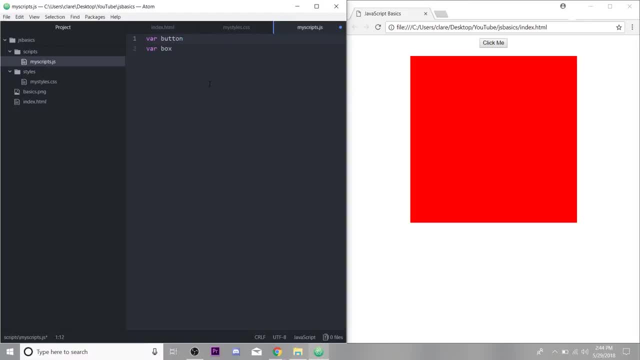 called box. okay, now i'm going to set this equal to. i could just leave it at this: javascript ends with a semicolon and then later we could do you know button equals and set a value in here. but i'm going to declare what this button is. 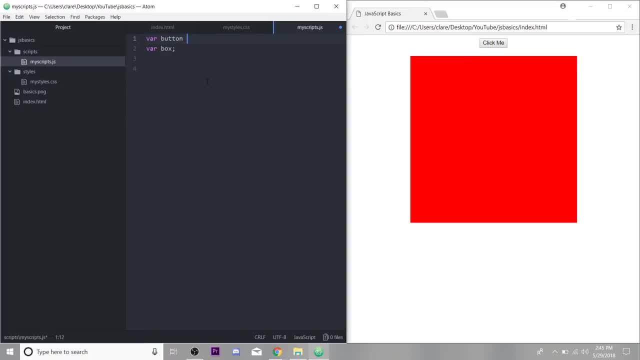 what's going to be inside the variable, what the variable will be right at the start. and this brings in something else that i want to talk about, which is property accessors, so kind of how selectors in css sort of dig into our document and grab what we want to style. 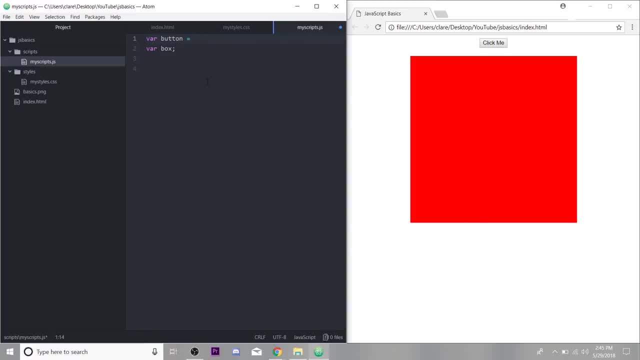 property accessors do the same thing with javascript, but they're done in the dot notation. so what i mean by that is document dot and then whatever we put after this is going to be what we're targeting here. so javascript has some methods which are just built-in actions that 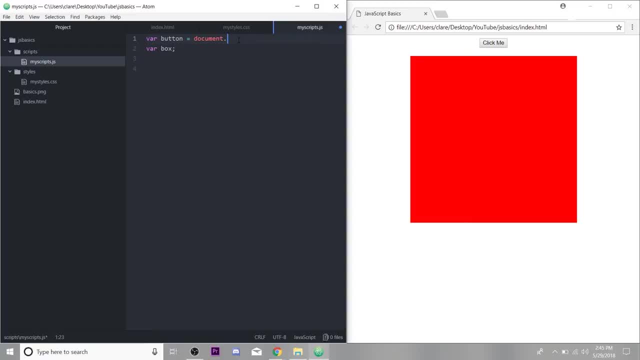 they do. they're very useful. i'm going to use the query selector method, and methods have parentheses after their name. same way functions do, which we will get into. so the query selector method: you just put in here what, what html element, basically what tag you want to grab. we are going to grab the. 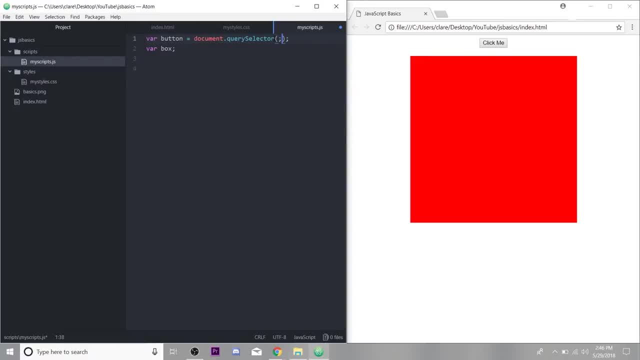 button right here, so we do query selector button. and now this button in html has been assigned to the variable button in javascript. this just means we can access that button and do something to it within our javascript code without typing out the whole selector. okay, and so for the box we're going to do something similar. 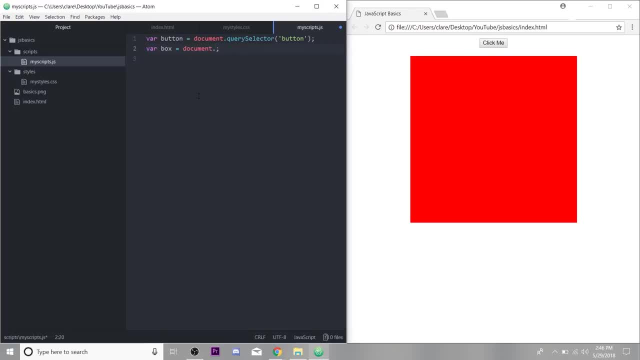 we're going to use a property accessor, but the method we're going to use instead of query selector is get element by id. this is another method in javascript that pretty self-explanatory. it gets the element in our html that it's linked to by its id. 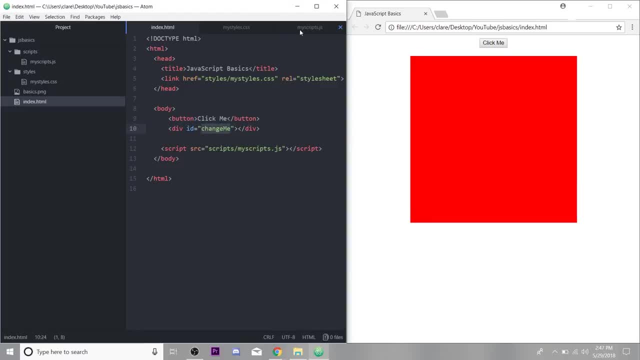 and remember: the div that is our box has the id of change me. so in the parentheses here of our method we just put change me. now this div is in our variable, in our javascript and we can do things with them. so what we want to do is, when we click this button, we want this box to change color. 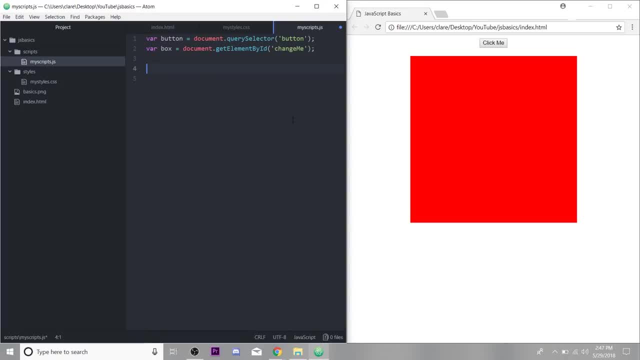 so we have to add an event first of all to the button. we just want to add the on click event. so when the button's clicked that's an event that. then we want the code to do something. so we're going to target a button again on click. this is the event we are adding. we want to set it to equal function. 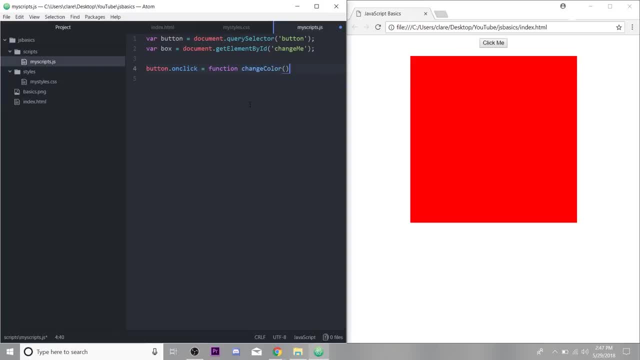 we're going to call our function, change color, and remember how i said, methods have parentheses after them. functions are always: this is the name of the function and these parentheses here make this a function. so we know we're calling a function and this will make sense when we're. 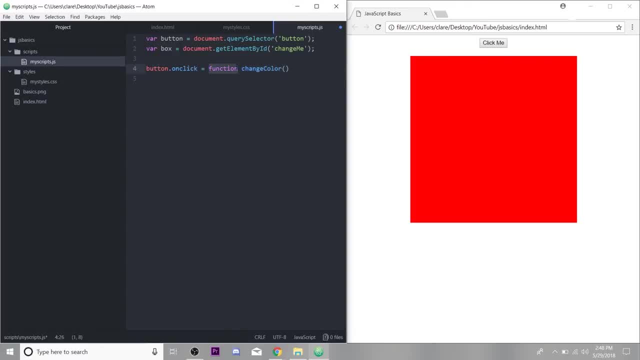 calling it somewhere else in the code, not right after declaring it. so we're declaring a function called change color and then after the name with the parentheses, we open and close our brackets and then the code we want to execute when we call the change color function go in here. so what we 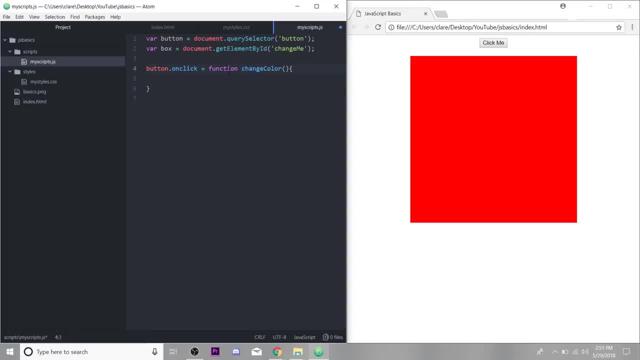 want to happen. when we click our button and run the change color function- in frogrun i am- and run the change color function is change the color of our box. so what we do in here is grab our box, access the property style. we want to access our background and set it to blue. 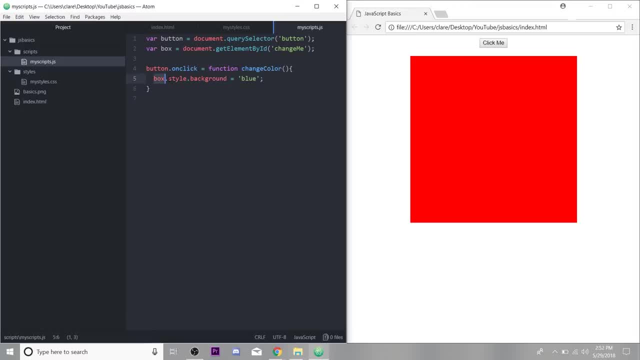 so box, and then this is getting into. if this were an html element, we could add a style property to it. and then, if this is getting into, if this were an html element, we could add a style property to it, a style property to it and set background to blue in it. so it's sort of. 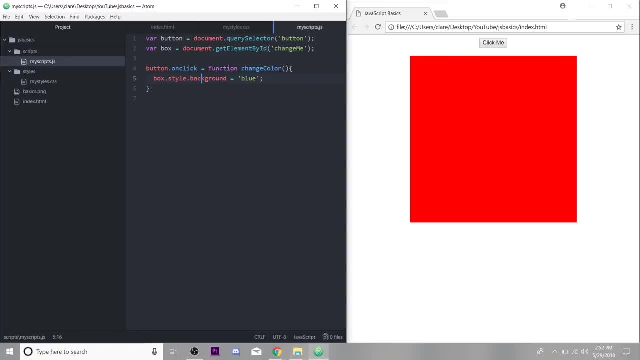 just without changing the markup, going in and changing something about it dynamically. so if we save this and refresh our page, I click the button and the box turns blue. so, but you don't have to have the on click in the JavaScript. which is cool about on click is you can set it to this property here, so we can. 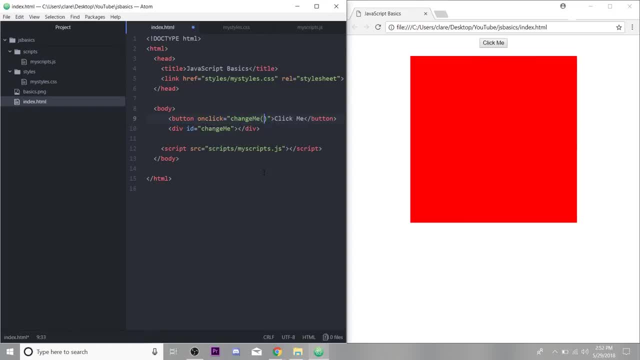 set the on click of our button to change me see, when we're referencing a function, that's all you have to do: the name of the function with the opening and closing parentheses. and if we were to set the on click here, we go into our JavaScript. we don't need to set it here and in the HTML. so what I would do is: 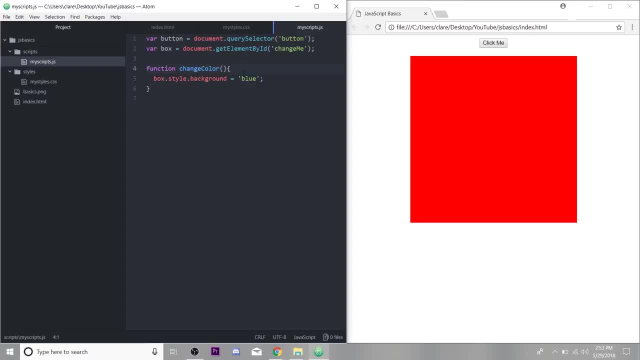 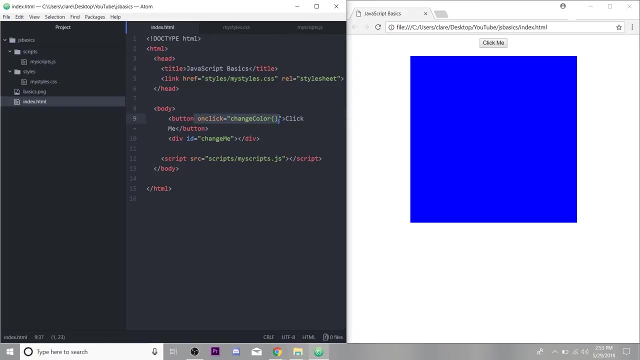 just remove the on click function from the JavaScript because we attach it in the HTML and now it should work the same way. oh, the functions called change color. so now it works the same way whether you are setting this event in the HTML or in the JavaScript. ok, so I mentioned conditional statements at the beginning. I want to 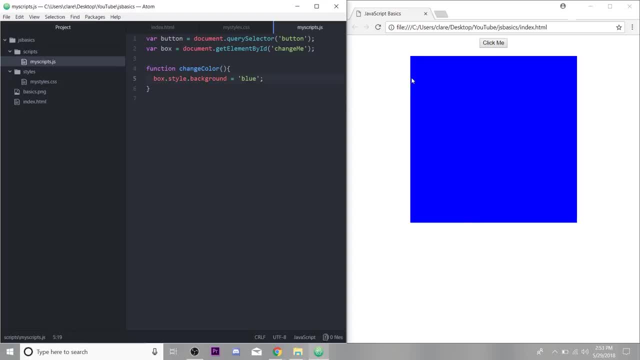 use a conditional statement in this change color function to check the color of the box, and then they'll be a kind of toggle effect. so the anatomy of an conditional if else statement is: if check this condition, execute this code. so if, whatever we put in here, do this, else do something else. so 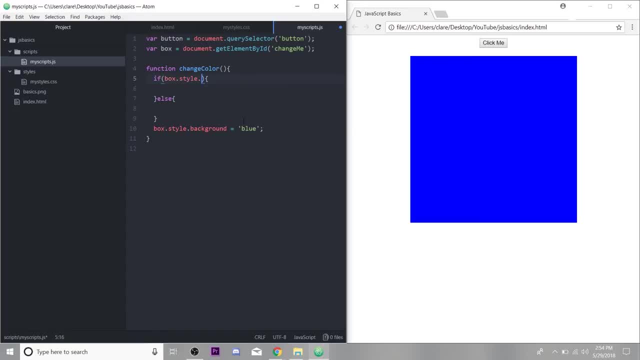 we are checking if box style background equals red, and you'll notice I did two equal signs here. this is a comparison operator that means equals, so it's two as opposed to just one. this would be setting something, so we're checking, not setting. we're using two. there are other comparison operators. 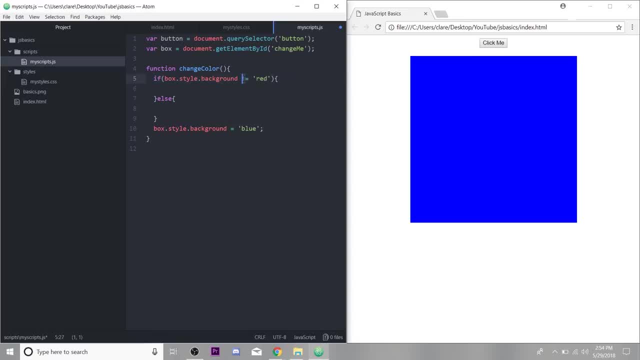 such as not equal to. the exclamation point is a negation symbol. there's also, you know, greater than, less than, greater than or equal to, less than or equal to, and this is identical, which is slightly different from equals. but we're just going to use equals for now, because we don't need to worry about the 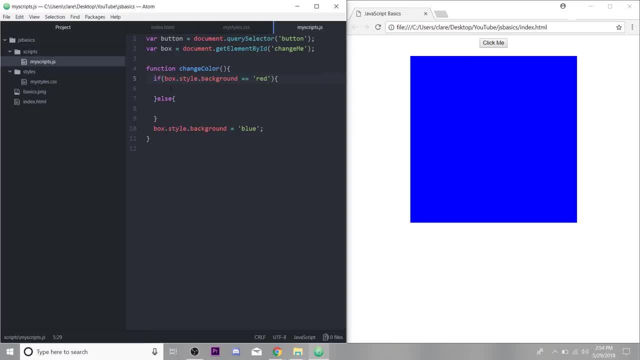 identical. so this conditional statement is checking if our box background is red, and if it is, we want to change it to blue. so I'm going to cut what we had already written and paste it in here. so if our box background is red, change it to blue, else let's change it to red. box style background equals because we're 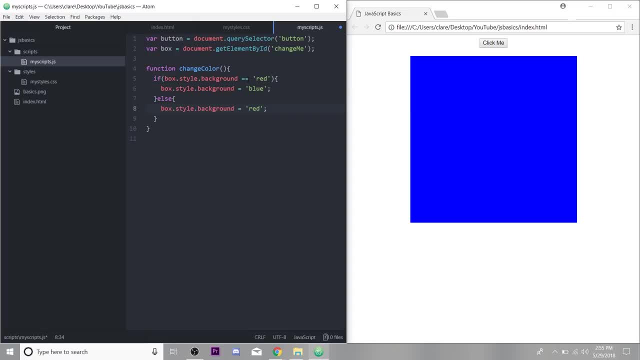 setting it. when we check we use our comparison operator of double equal sign. when we're setting, we just use a single. okay, so if we save this and refresh, if it's red it changes to blue and now it's blue. if we click it, it should check. if